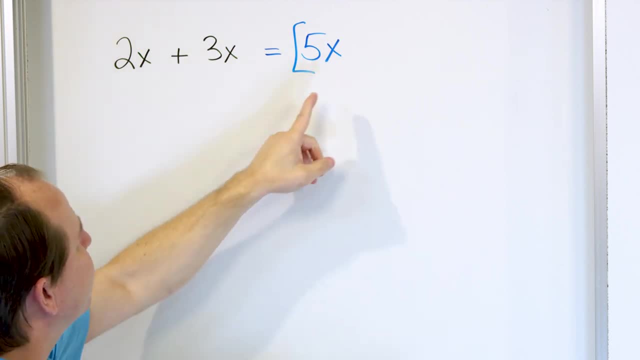 hamburgers means I have to have 5 hamburgers. So a lot of students aren't sure why they have to have an x in the answer. Why isn't the answer just 5?? Well, the reason is because you're not just adding 2 plus 3.. You're adding 2 of these things. You're adding 2 of these things. You're. 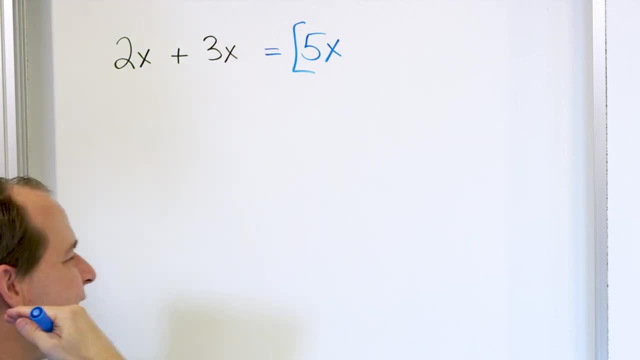 adding 2 of these things plus 3 more of these things, And it's easier in your mind to think of them as bananas or something. coconuts: 2 coconuts plus 3 more coconuts, So I have a total. 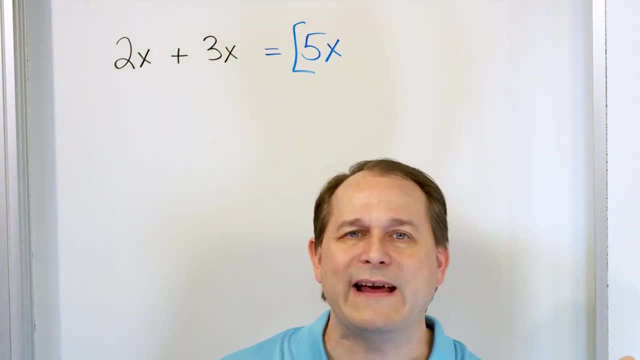 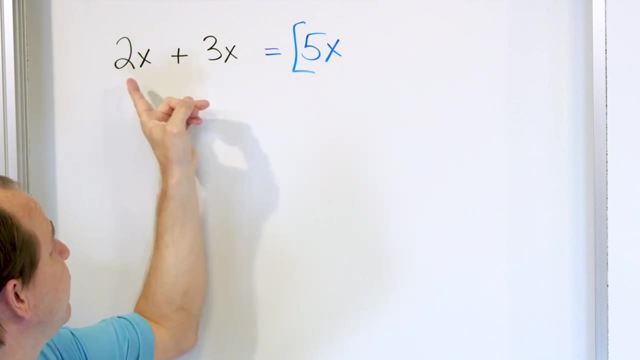 of 5 coconuts. right, And that's why the terms have to match, because you really can't add coconuts to giraffes. If the variables were different, like if this were 2x plus 3y, then I would not. 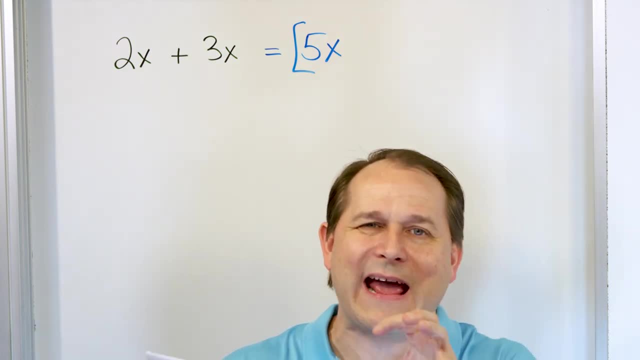 be able to add them. You can't do anything with that, because you can add giraffes to coconuts, I guess, but they're different and they're not the same thing, So it doesn't make sense to add them In order to add or subtract things in. 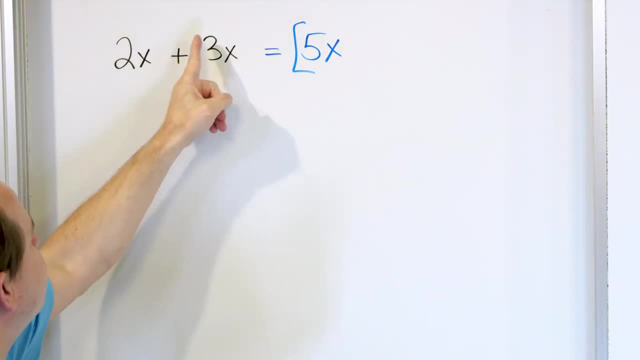 algebra. the variables have to be the same and also the exponents, which in this case both are just little exponents of 1 that are invisible there. They have to match as well. We'll talk more about that a little bit later. Once the terms are matching, we say that these are like: 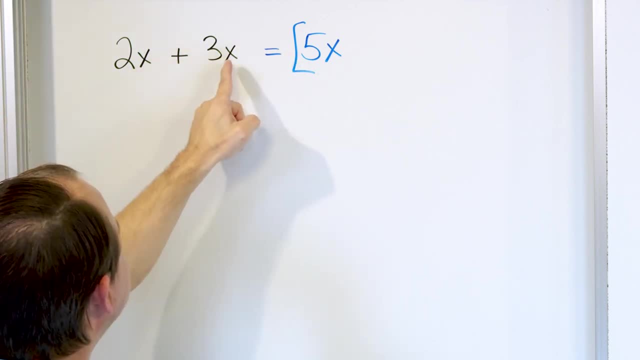 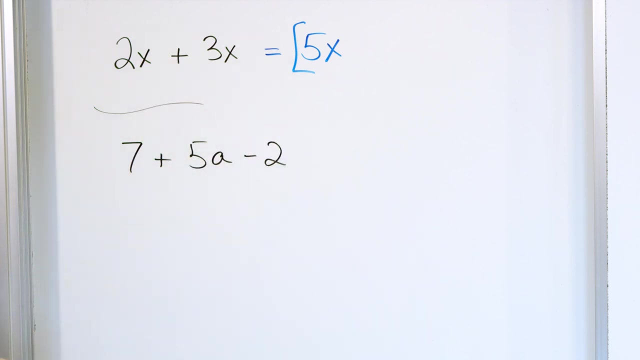 terms, And when we have like terms we can just add the numbers and then the x carries to the end, because 2 coconuts plus 3 more coconuts is 5 coconuts. All right, let's take a look at problem 2.. Let's say we have 7 plus 5 times a minus 2. How do we? 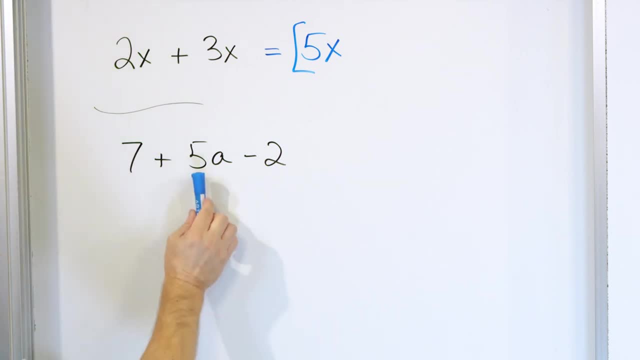 simplify this expression. Well, what are the like terms? We have one term that has a variable, So this is like 5 bananas, right? But then this term has no variable. It's not a banana term. And this has no a as well. It has no variable, So it's not a banana term either, right? So because of that, 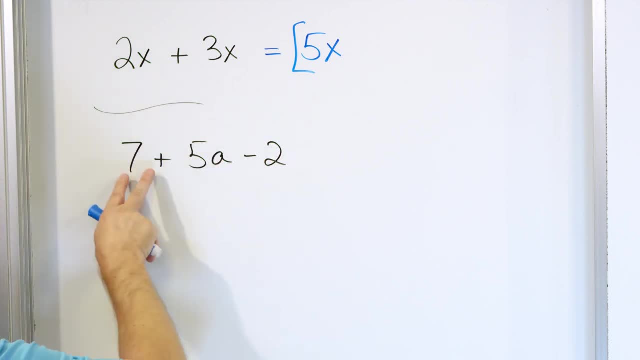 we can't really add the 5a to either of them, Because this is different than this and this is different than this. So we just can't add these. But the numbers of course can be combined, because there is no variable here and there is no. 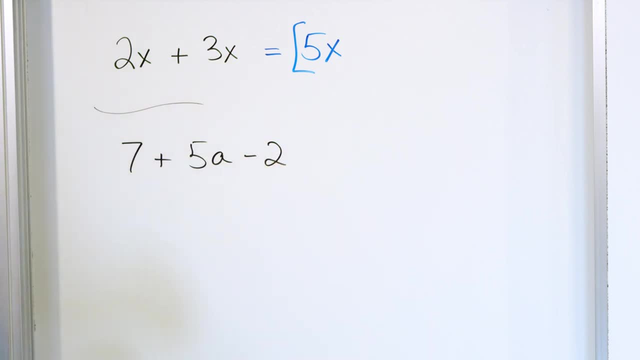 variable here, So the numbers are like terms. That works just fine. Now, after a while you won't have to do this, But in the beginning it helps for us to move things around right. So here we can just say that this is 7 and we know we're going to add the number, So we can take this: 2. 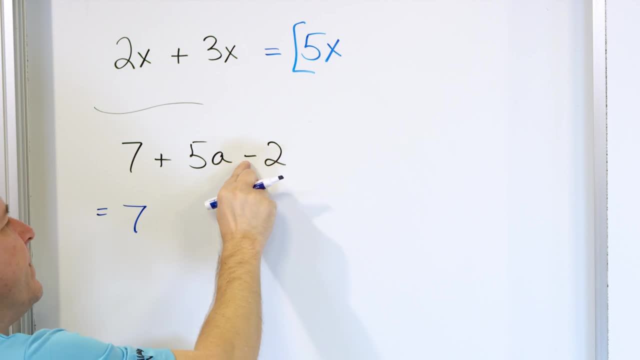 and we move it over here. But when you move terms around the minus 2, the little 7, we're going to add the number. So we can take this 2 and we move it over here. But when you move the sign or the operation right in front, it's attached to the 2.. It's attached to whatever. 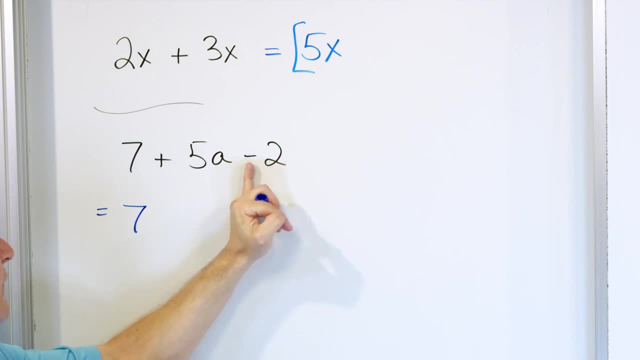 you're moving. Everything in life has a sign. The sign of this 2 is negative because there's a negative in front. The sign of this 5a is positive because there's a positive here. And the sign of the 7 is also positive even though it's not there, because the positive is invisible. 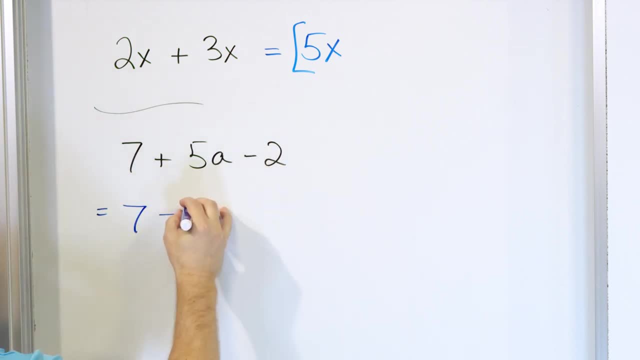 but it's there. So when we move this 2 next door, we have to move the minus sign with it. That's what I'm trying to say. It's attached, It's like just stuck to it and it goes with it, And then 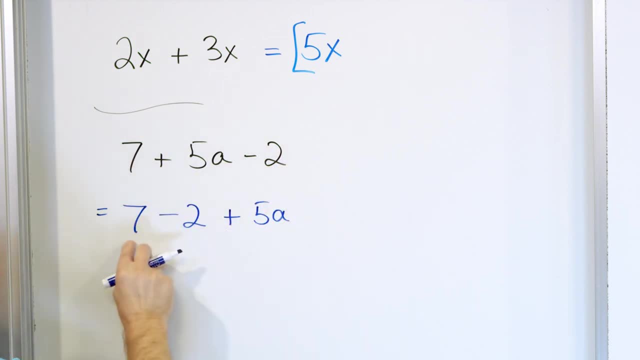 the plus comes from here, And then the minus sign comes from here, And then the plus comes from here, And then the 5a here. Now that they're written next to each other, it's very easy for you to see that we can subtract 7 minus 2 to get 5 plus 5a. Now you might want to add these You. 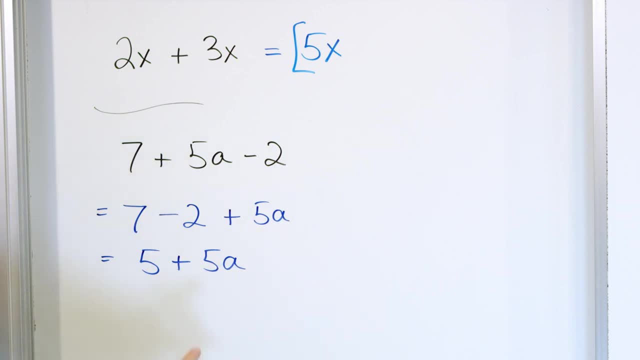 might want to combine them and write 10 down or something, But you can't, because this is like five horses plus five nothings, five buffalo or something, And it doesn't make sense and you can't combine them. Now one last thing: When you write the answer, usually you write the terms that have: 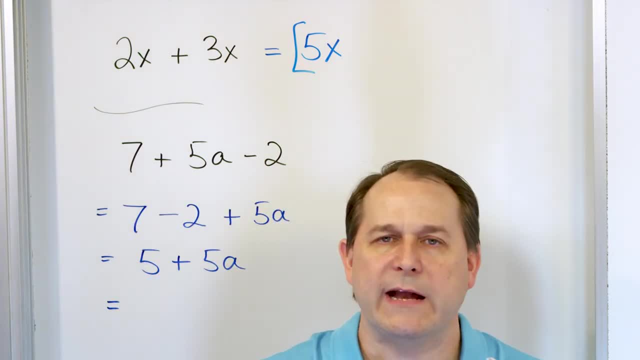 a variable first, And you know when you add things you can't just write the answer first. You can change the order of addition right. 2 plus 3 is 5. And 3 plus 2 is also 5.. So these are. 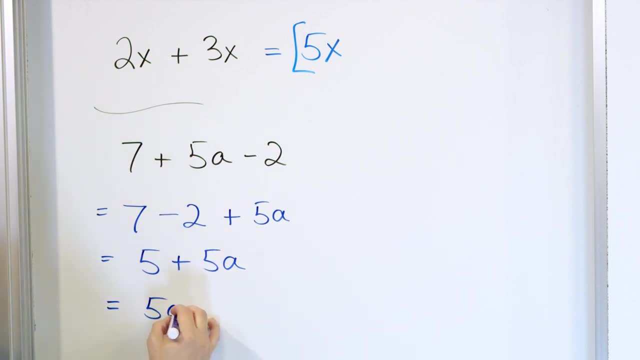 added together. I can flip the order and it doesn't change anything. So I can write this as 5a plus 5.. That's the same reason that I was able to take this minus 2 and move it around, Because when you add or subtract things, as long as you grab the sign with whatever it is, you're moving. 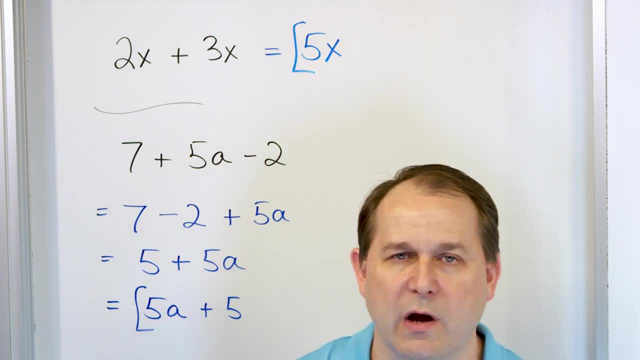 then you can rearrange things as much as you want to in your addition and subtraction. It won't change the answer. So the answer to this is 5a plus 5.. Now you have to get used to seeing your answers to have a plus sign in there. 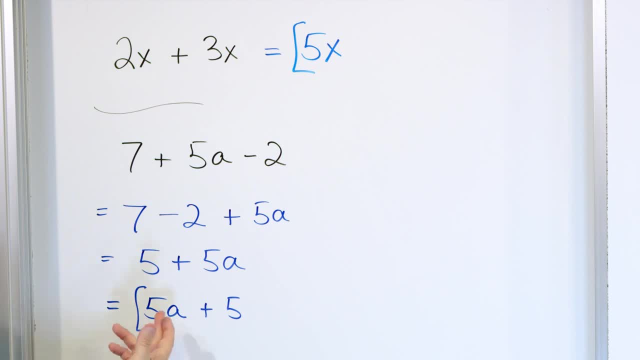 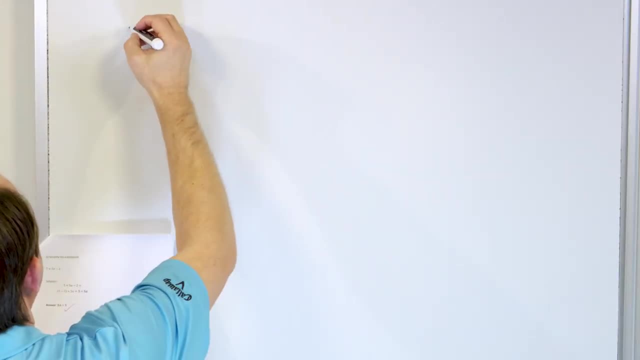 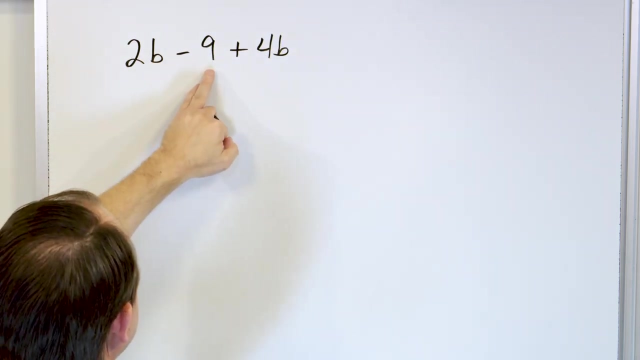 And you want to, in the beginning, combine them, But you can't, because this is a totally different kind of term than this, because this has no variable. All right, let's see another example. What about 2 times b minus 9 plus 4 times b? Well, we have a number here, but we don't have any other. 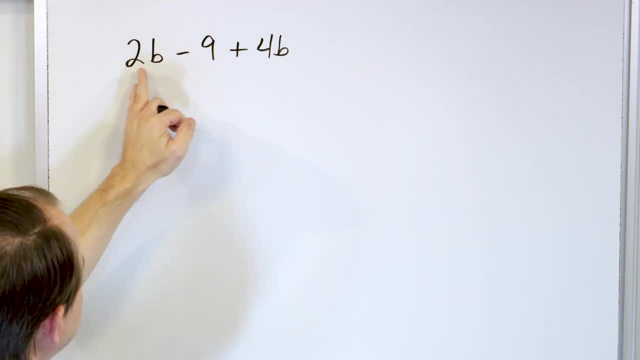 numbers by themselves, So we can't combine the 9 with either of these things. But we do have a 2b and we have a 4b, So this could be like a 4b. So this could be like a 4b. So this could be like a. 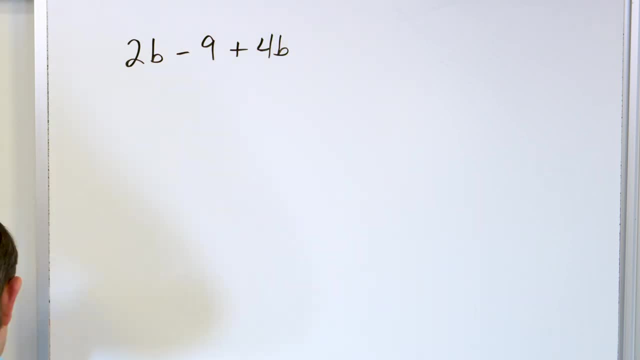 2b, So this could be like a 4b. So this could be like two buffaloes and four more buffaloes. Now let's spend a minute to write. these guys right next to each other. We have 2b from the problem. 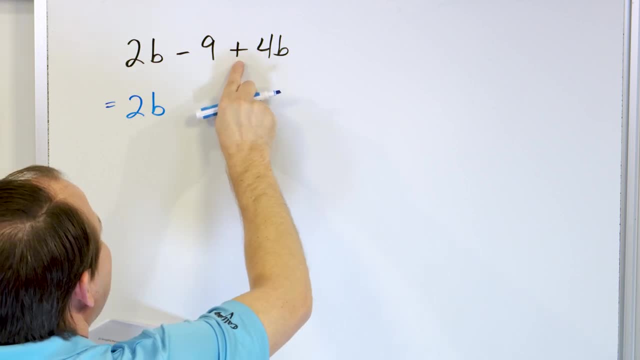 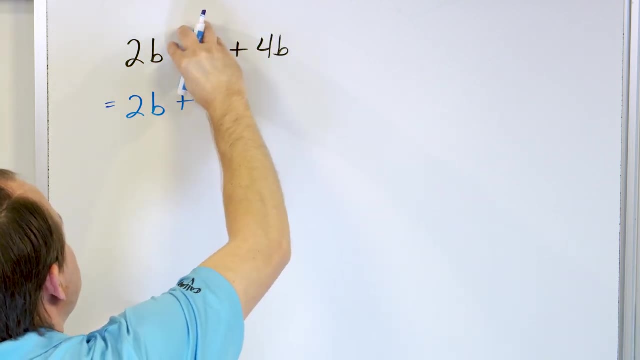 statement And we want to combine it with this. We can move it next door And the sign that is attached to it is a plus sign because it's stuck right in front, So we can move it right next door, And then the minus 9 has to go with a minus sign at the end because the minus sign is stuck to the 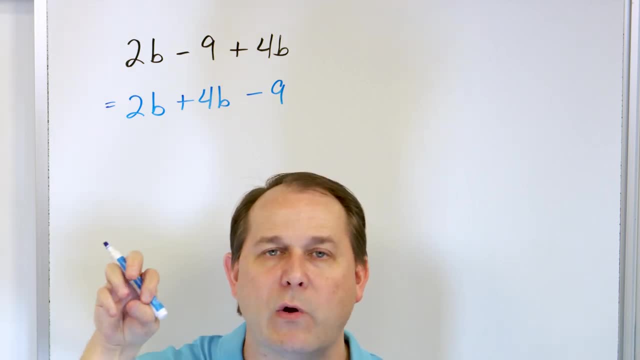 9. So when you're arranging terms you have to grab the sign right in front. It is attached to it. It very important. That's a great way to get screwed up when you move things around and you don't grab the signs also. So the plus four B goes here and the minus nine goes here, And then we can see. 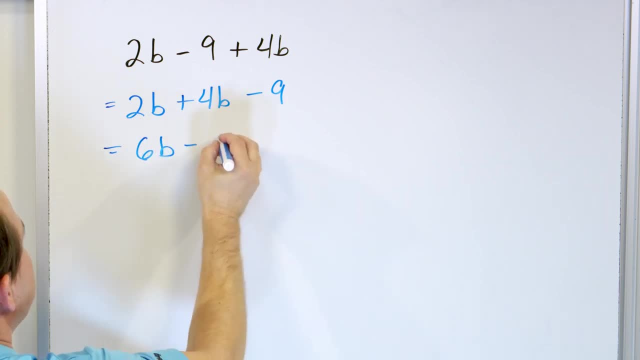 more easily: two plus four is six B's minus nine, And we typically want to write the variable term first in any number terms, constant terms later, And so we'll say six B minus nine. Now you might want to add or subtract this as much as your heart is telling you to do it. You can't, you can't do. 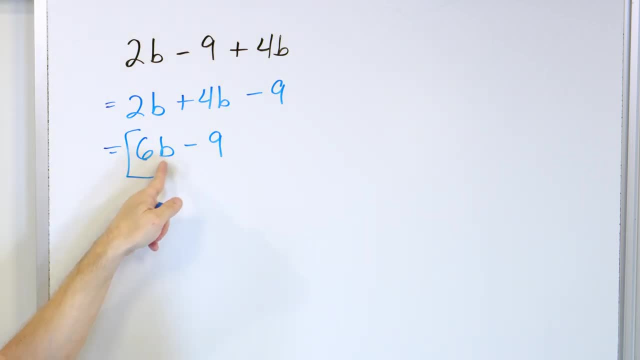 it because this is six. you know six cars, and this is nine minus nine. I don't know what it is, but it's not cars, It's different, And so you cannot subtract them or add them. You have to leave it like this And you have to get used to seeing that, because up until this point in math, 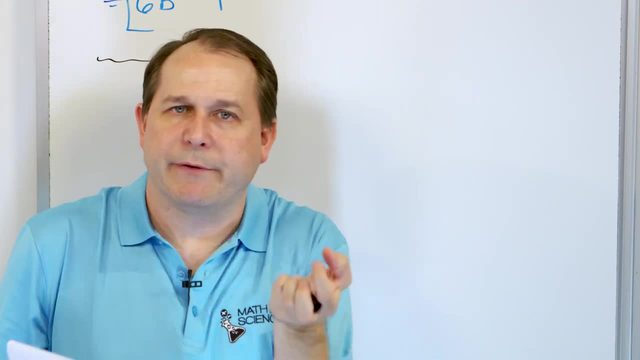 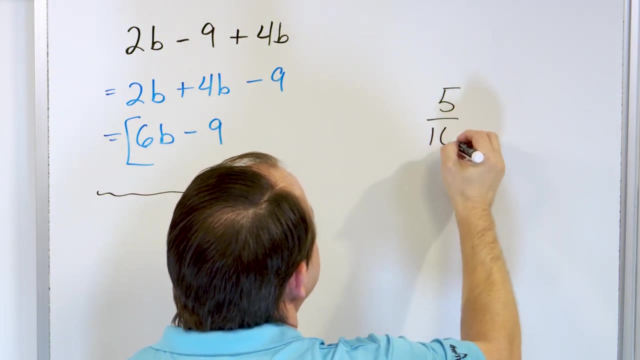 you know we're used to getting numbers as the answer. Now let me, before we go on, let me just show you what we're really doing here. If I tell you that you have the fraction five tenths, this is five slices out of. 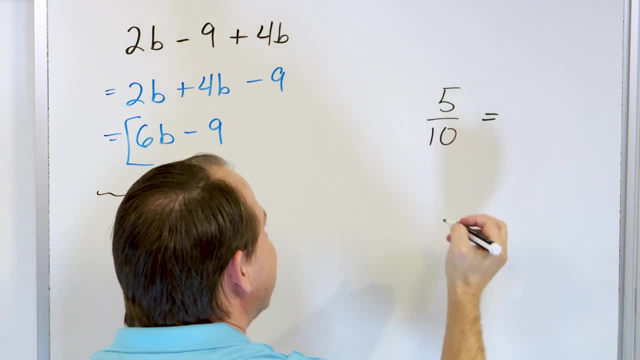 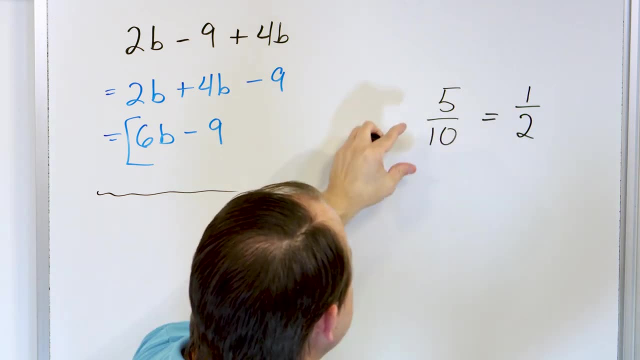 10. 10 slices in a pizza, And you know that if you actually have five out of 10 slices, it's the same thing as one half, right? Because I can divide the top and bottom by five and I'll get one half. You know that, And you know that this fraction means exactly the same thing as this. 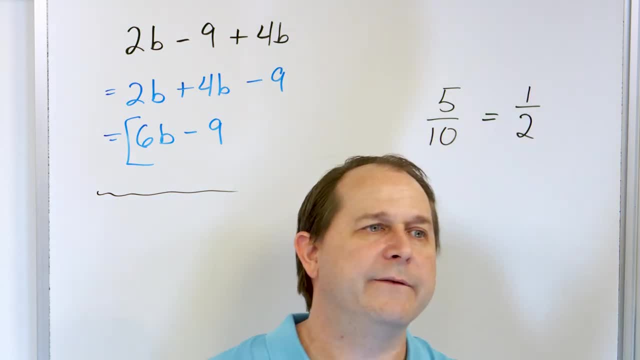 fraction, They look completely different. If you ask a five-year-old what this is and what this is, they're going to tell you they're different. The numbers are all different, but we know what fractions are And we know that they actually are exactly the same amount of pizza, What you need to. 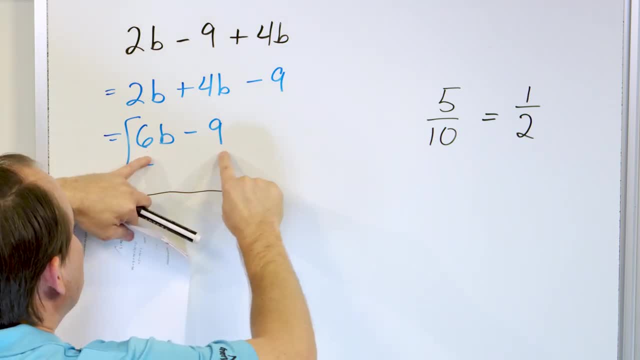 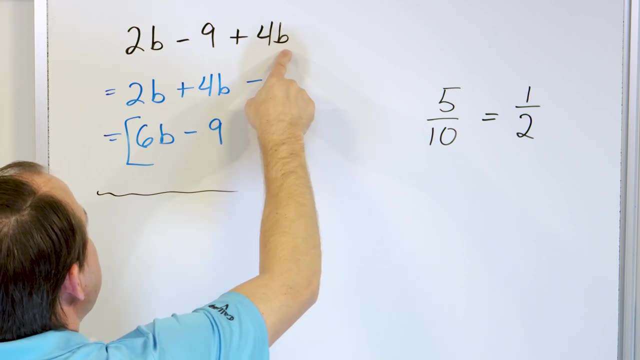 realize when you're doing these problems is that the answer you get looks totally different than what you started with, but they are exactly the same thing. If I put numbers in for B, like B is equal to well, you just put B is equal to zero. 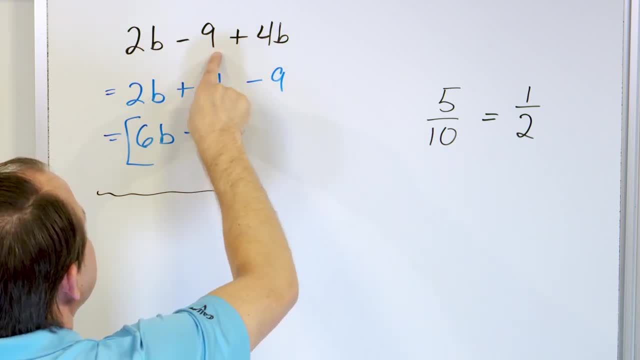 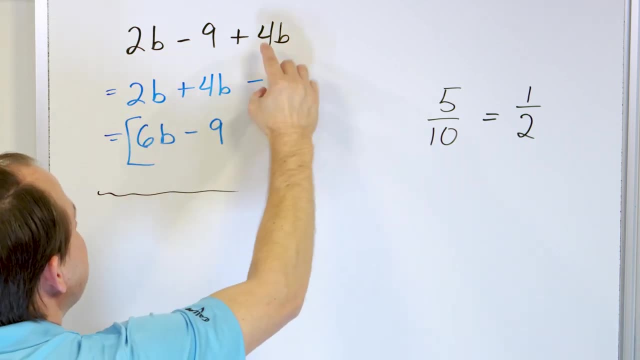 then this will go to zero and this will go to zero and you'll have negative nine. But if I put B is equal to zero here, this will go to zero and you'll still have negative nine. This expression looks different, but it's exactly the same answer for any value of B that you put in there. It's the. 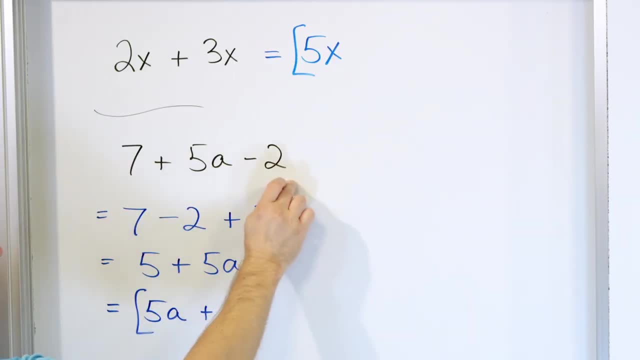 same thing. This looks totally different than this. The number here is different, but it is the same thing. If I pick any number I want for A and put it in here, I will get the same answer here as I calculate here, just like in the fraction case. So when you're getting these things, it looks like you're getting. 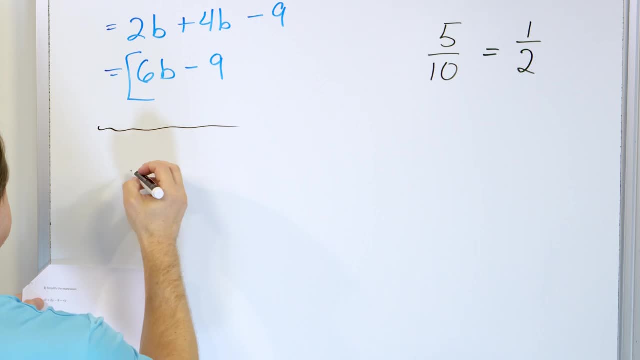 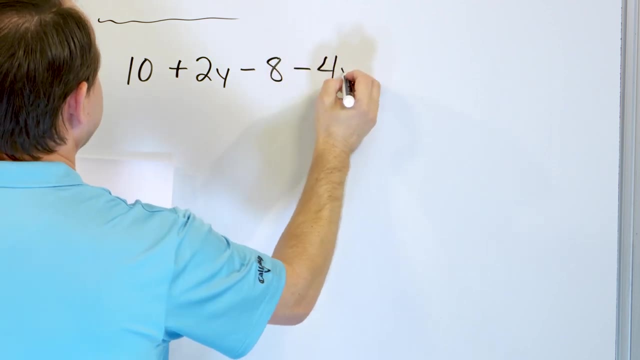 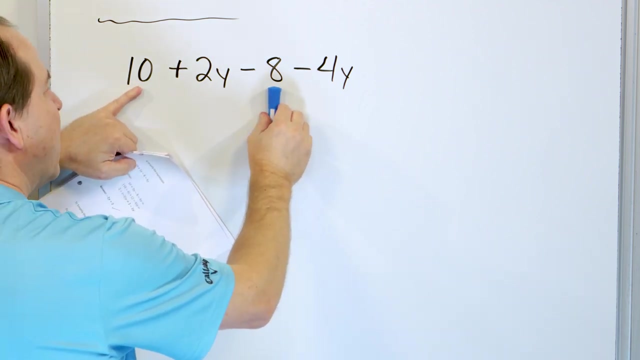 things that are totally different, but in fact they're exactly the same. Next problem: 10 plus two times Y, minus eight minus four times Y. All right Now, what terms are like terms? Well, with the 10 and the eight, these are just number terms, constant terms, Those are like terms. 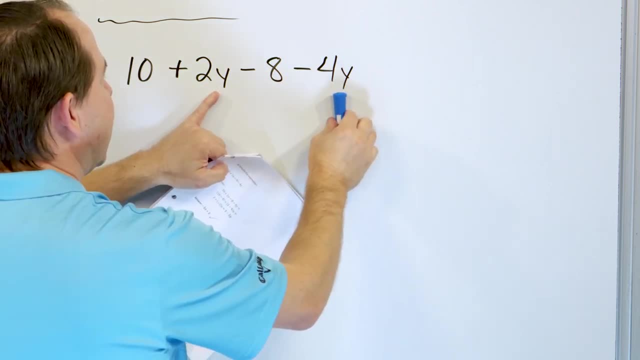 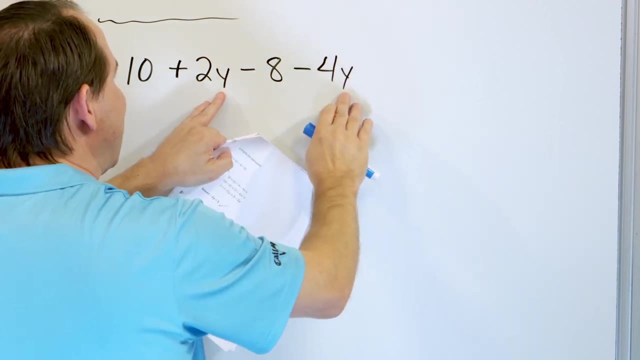 We can combine those And then the two Y and the four Y. these are like terms because it has the same variable And also there's an invisible exponent of a one here in both cases. So they match completely the variable and the exponent. So let's take a minute and combine these in a way. 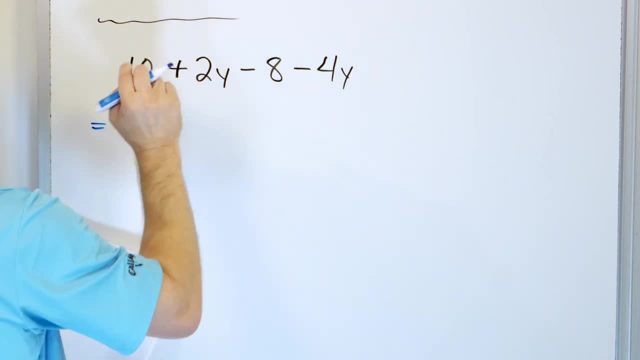 that makes sense. So let's take the minus eight and move it next door to the 10.. So we'll have a 10 here. Remember, the number has a sign attached to it. It has to change, So let's take the minus. 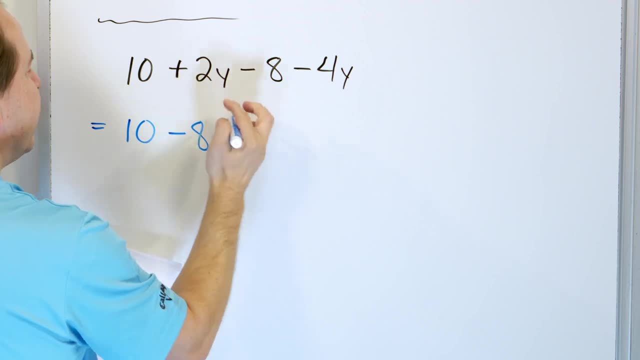 eight and move it next door to the 10.. So let's take a minute and move it next door to the 10.. So we move the minus eight there. Then we have a plus two Y. That's written right from here And. 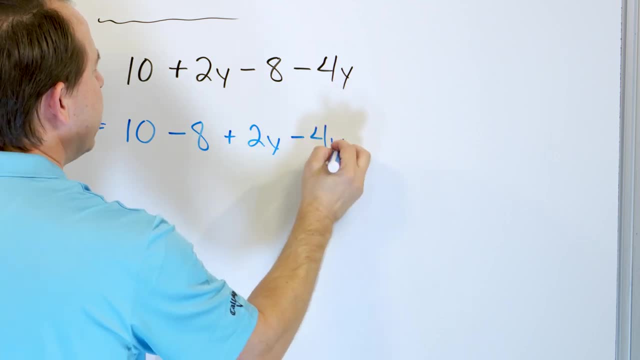 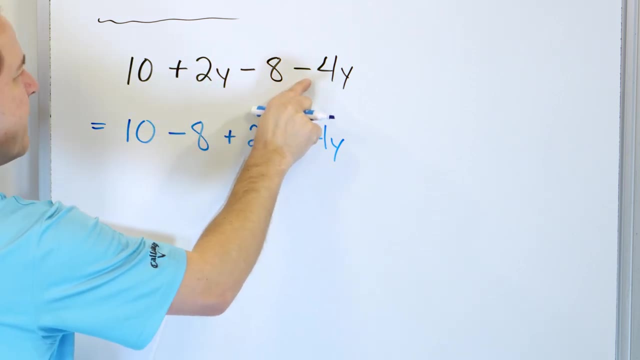 since we moved this, the only thing left here is minus four Y. You see what we did? All we did is we take the minus eight and we put it right in between here, So we have 10 minus eight, and then the plus two Y, and then the minus four just stay in place. But now the terms are right next to each. 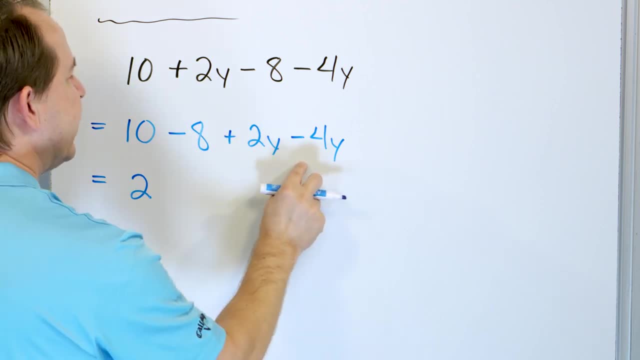 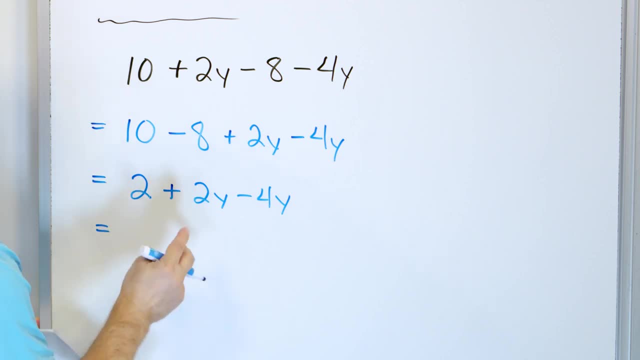 Y minus four Y. Now we'll combine these Here. we have to think We have two Ys minus four Ys. So what we have to do is we're going to basically subtract the numbers and the Y is going to come along in the answer. It's like two horses minus four horses: It's the same animal. So we can. 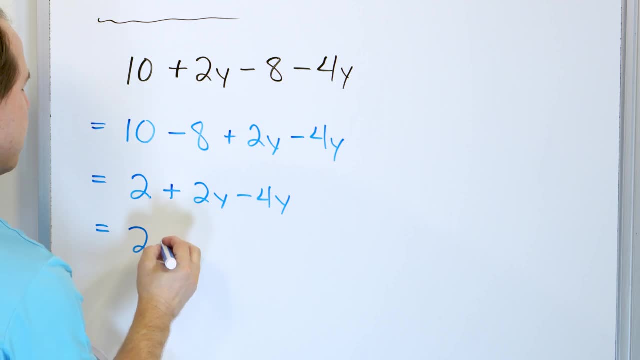 subtract them. What is two minus four? Two minus four is what Minus two? Because remember, when you start with a small number and subtract a big number, you can just reverse it and say four minus two and then put it back together. So we have two Ys minus four Ys. Now we'll combine these Here. 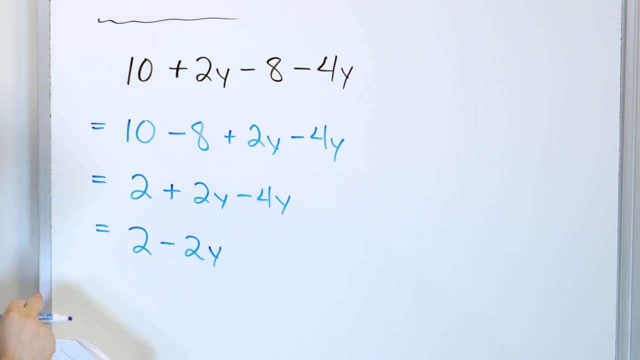 we have two Ys minus four Ys. Now we're going to subtract them. So we have two Ys minus four Ys. Now we're going to put the negative on there. But since we have a variable there, the variable has to. 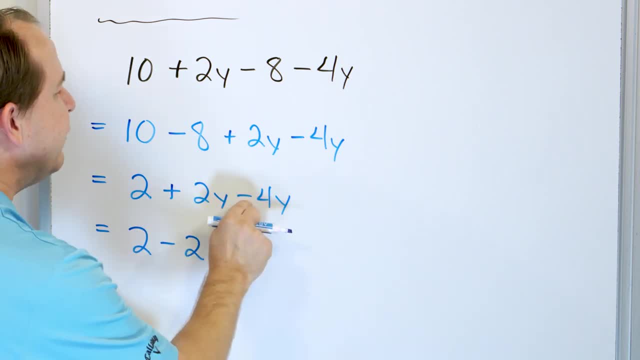 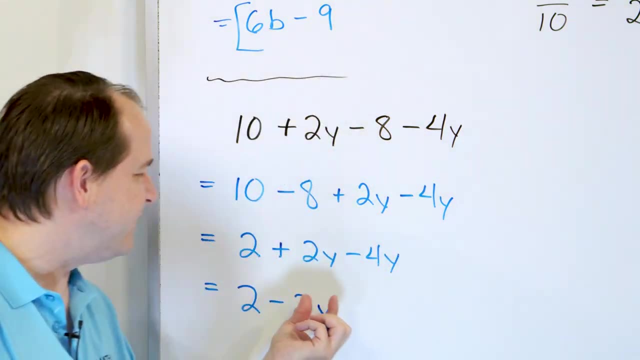 travel. If you think about it, if you really did have two horses and you subtract four horses from it, then I only had two to begin with. So I give those away, but then I give two more away. I must be in debt by two more horses. Two horses minus four horses gives me a debt of two horses I owe. 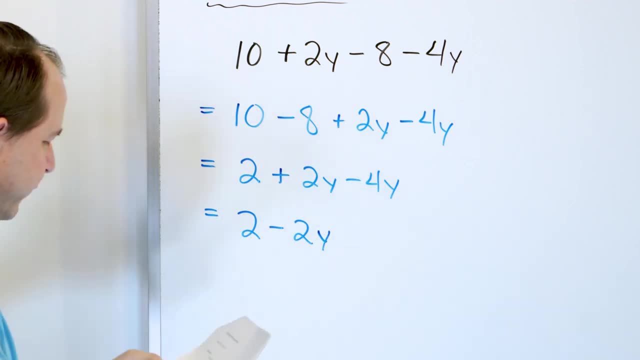 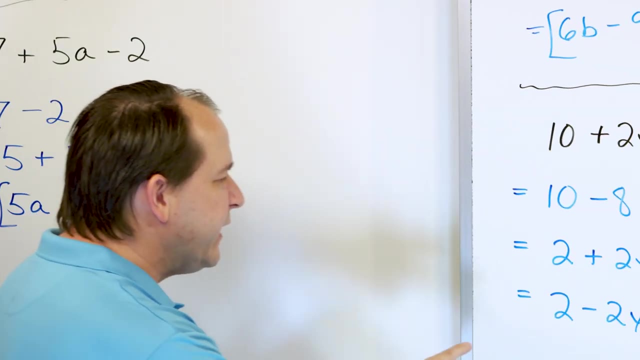 somebody The number minus. this is the answer Now. usually we want to write the variable term first. Usually we want to write the variable term first. We want to write the variable term first. So here we have the number first and we generally want to rearrange it. The negative two, Y, has to. 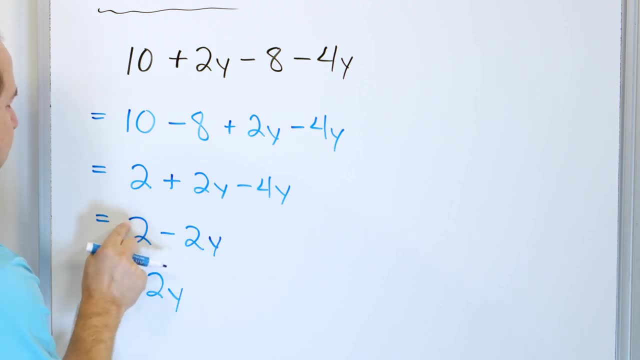 come out in front. The negative sign is attached to this and the two has a plus sign attached to it. So really, this is the best way to write it. Either one of them is correct, but usually you want to write the term with the variable first and then the number term at the end. negative two Y. 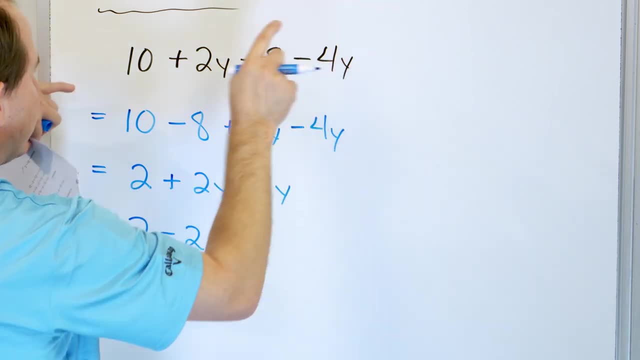 plus two. This thing looks completely different than this. I agree with you, They look different. But if I put a number in for Y, any number, negative, positive, zero, any fraction, anything, and put the same number in here, I will calculate the same answer. 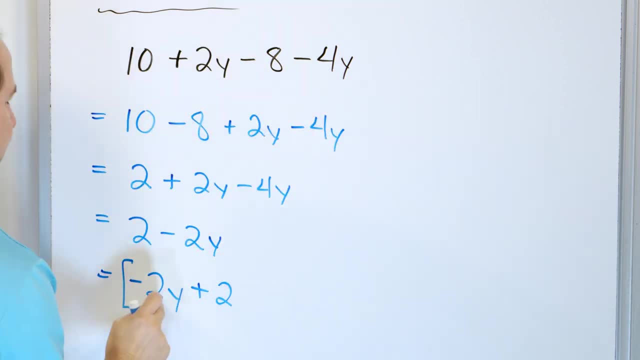 because this is just a messier way of writing this. This is a more simplified expression, And the stuff that we're doing here is very important, because when we solve equations, we're going to be doing this kind of thing for every single problem. Now, what about eight times? 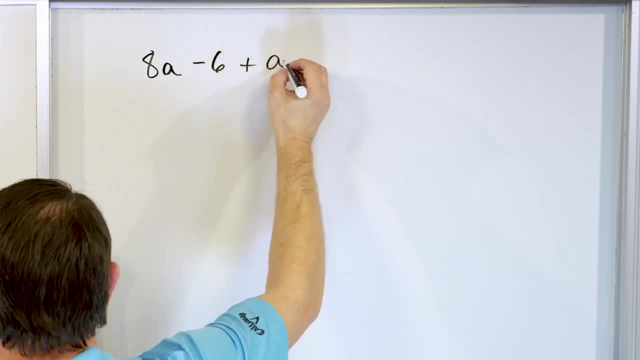 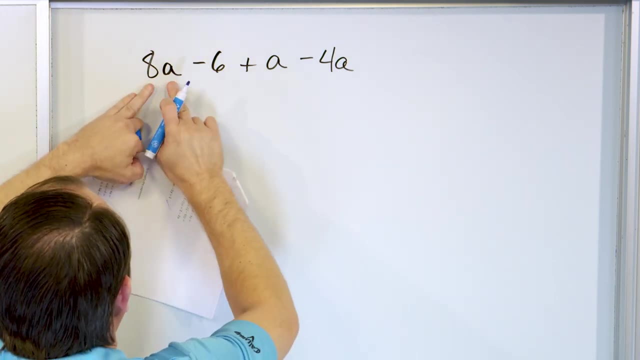 A minus six plus A minus four A. We want to simplify this expression. So let's group the terms that are lost. Let's group the terms that are lost. Let's group the terms that are lost. So this is a eight A's, This is an A. There's an invisible one in front, So it's a like term. And 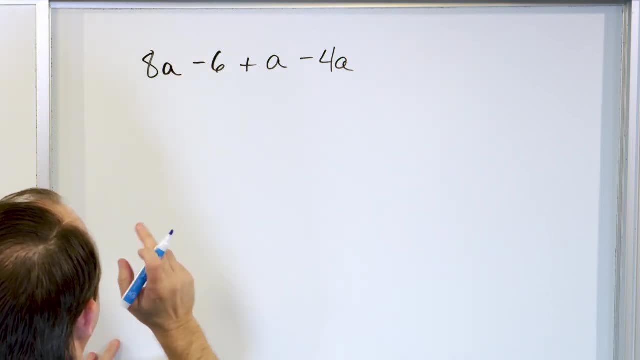 then this is minus four A. So all the A's are all correct. So they're all the same type of term. So we're going to have eight A. We're going to move this to the end. We'll just move this next door. 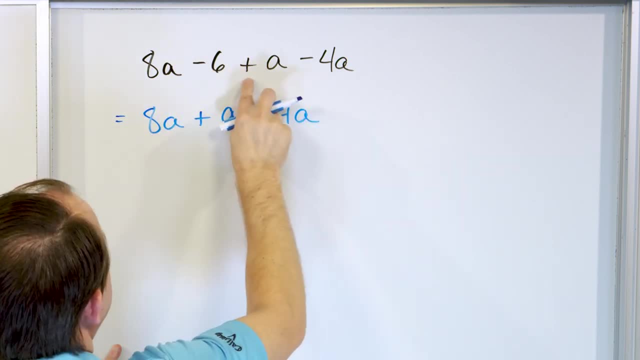 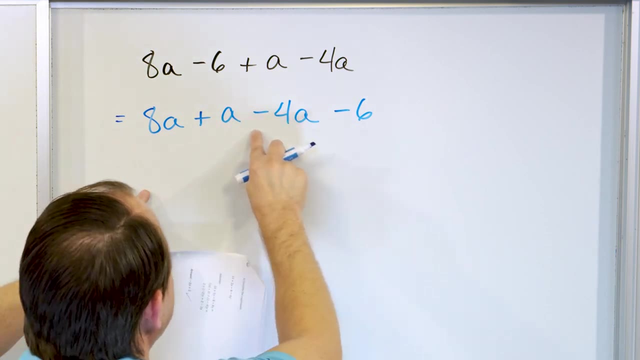 plus A minus four A. All I did was say this: plus this minus this, This minus six, because the minus goes with it. I'm going to move it to the end. I can rearrange my terms and put all my like terms together. This one, I'm going to put it in the middle. I'm going to put it in the middle, I'm. 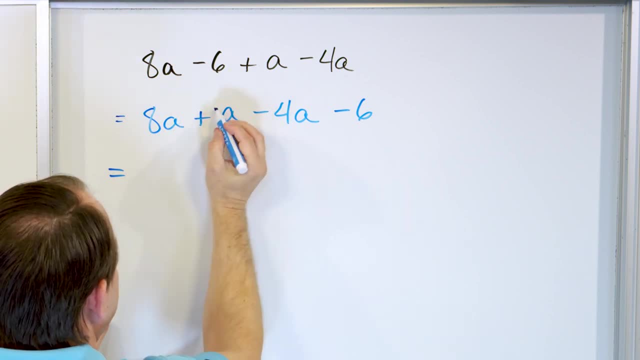 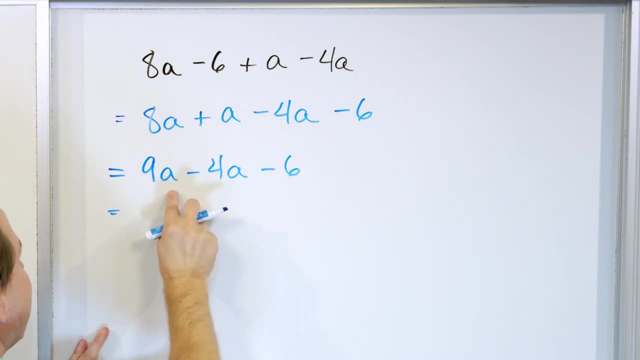 going to put it at the end: Now, what is eight plus one- Because there's an invisible one here- That's nine. So I can write this as nine A minus four, A minus six. And now again I have like terms. What is nine minus four, Five, So five A, And so the answer is five A minus six. Now, 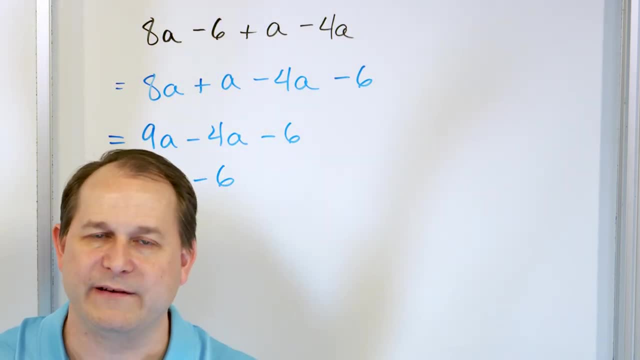 you have to get used to the idea. when you're adding variable terms together or subtracting, the variable just comes along for the ride And the best way to think about it is: nine cheetahs minus four cheetahs Is five cheetahs. That's why the variable comes down with it. Students like to do all kinds of. 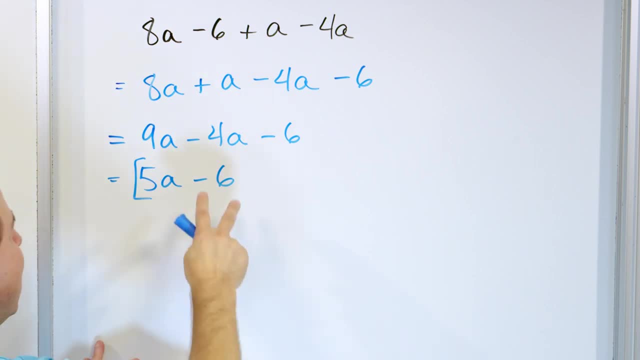 things with this variable. But what really has to happen when you add or subtract it is, it just gets, comes along into the answer, And these terms are different because there is no variable here. So you're done, And that's as far as you can take it. Five A minus six. 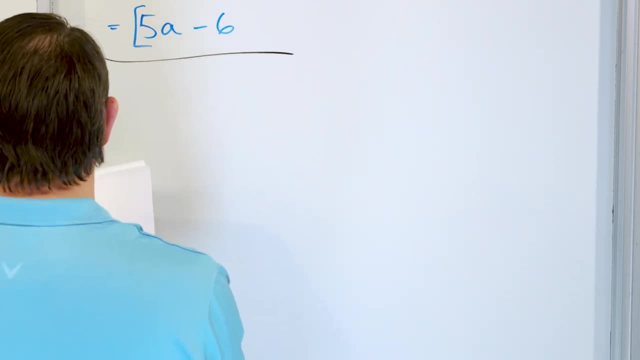 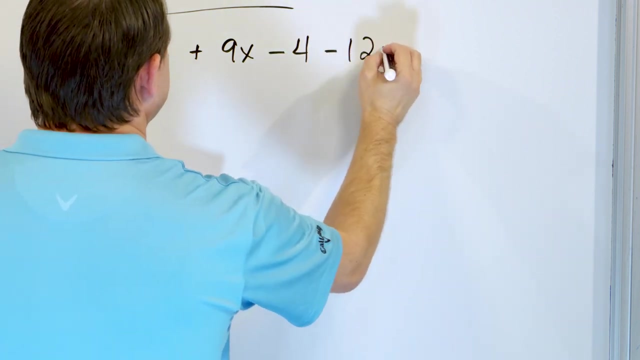 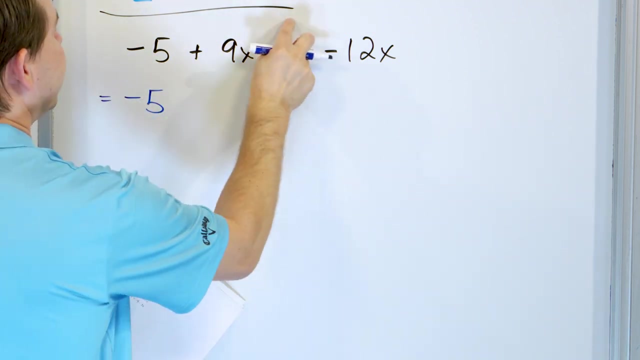 All right, We're going to speed up just a little bit, as we have the general idea here. What about negative five plus nine times X, minus four minus twelve times X? Let's rearrange terms. We have a negative five here. I'm going to take this negative four. 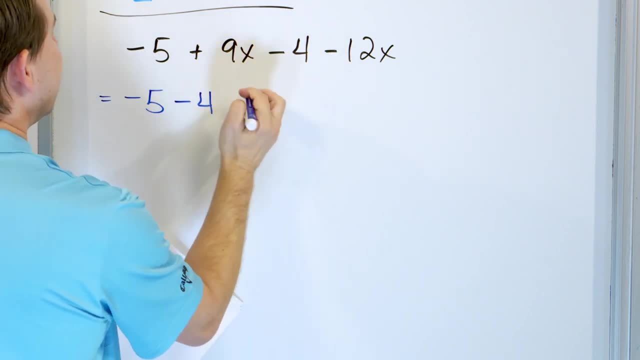 which is a like term, and write it right next door. The negative goes with it. The plus nine X is going to stay in play place, And then the minus twelve X has to come right here Again. the minus four- the minus sign- travels with the four. The plus travels with the nine X, The minus travels. 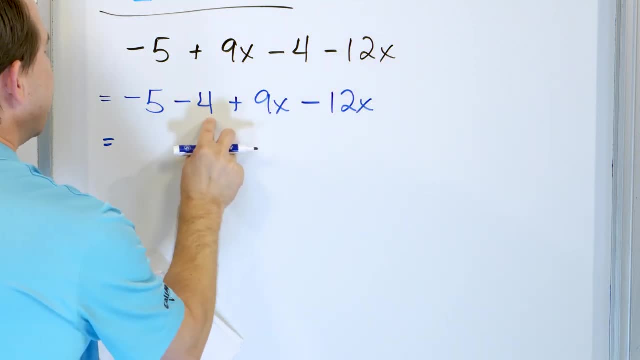 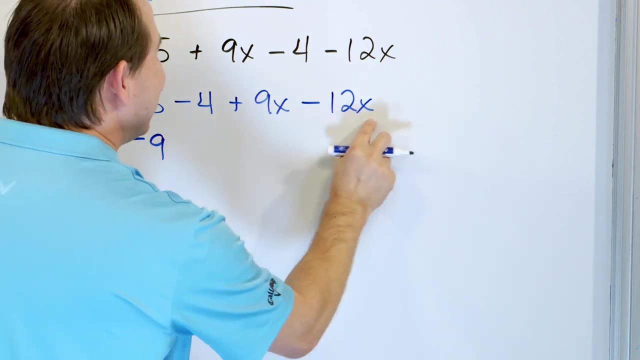 with the twelve X. Now, what is minus five, minus four? If I start with negative five and I subtract four away, it comes out to negative nine. So I'm going to subtract four, I'm going to subtract four, And then we can add these terms as well, But we have nine minus twelve. The X's are the same. The 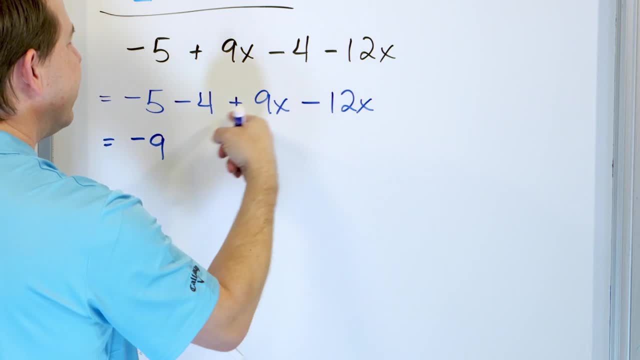 exponents are all the same, So these are like terms. What is nine minus twelve? Well, we subtract the other way: Twelve minus nine is three, And but because it's backwards, nine minus twelve, it's really negative three, And so it's negative three X, So you can think of it as nine plus a. 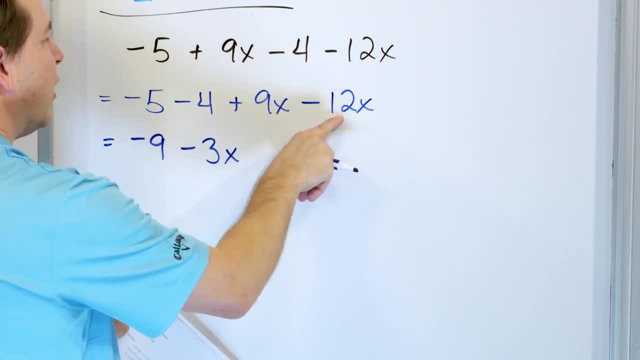 negative twelve. If you want, you subtract them and the sign goes with the larger absolute value. That's why it's a minus sign. It just travels along. If I have nine horses and I subtract twelve horses, well I owe somebody three horses, And so it's negative nine minus three X. Now usually we want to write the variable. 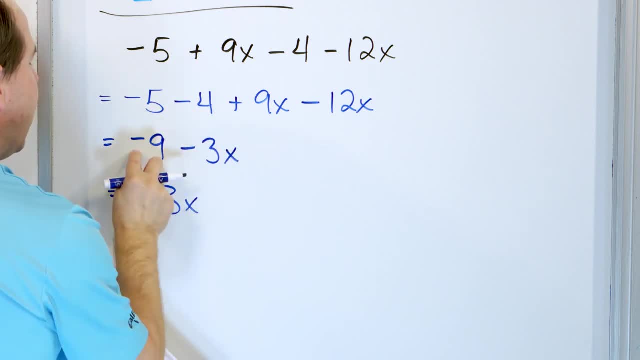 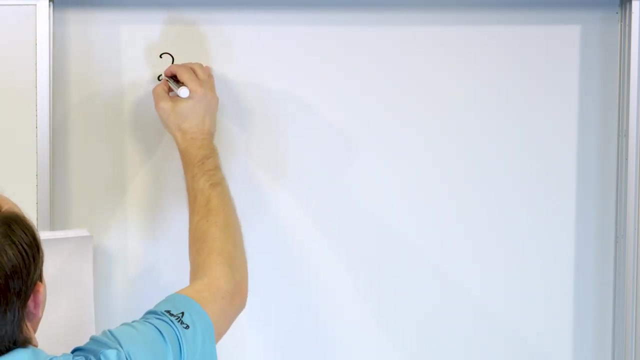 term first. So this one we're going to write first negative three X and then the minus travels with the nine. This is the best way to write it: Minus three X, minus nine. This is correct. This is better. All right, Moving right along. Let's take a look at something a little larger: Two times B. 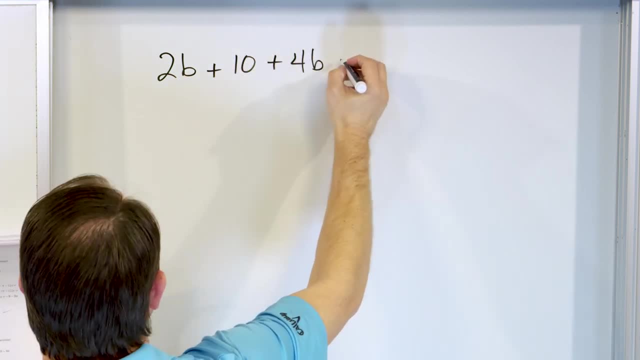 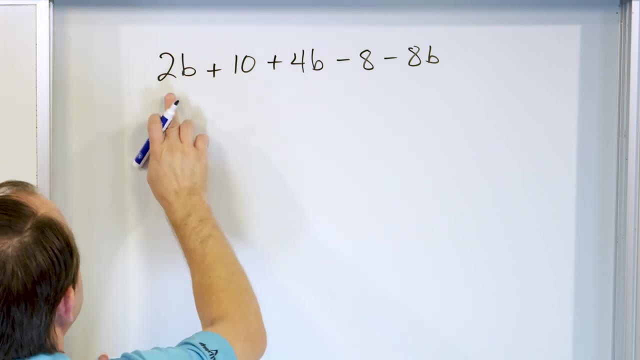 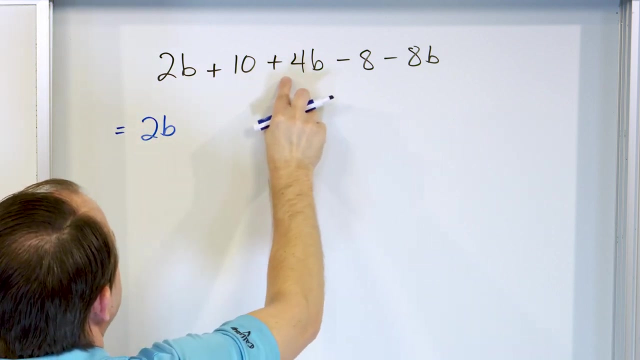 plus four times B, minus eight, minus eight times B. All right, Let's group all the like terms. This is a like term. This is a like term. This is a like term because all the variables are the same. So two times B, plus four B, and then minus, minus goes with it Eight B, And then we have the plus. 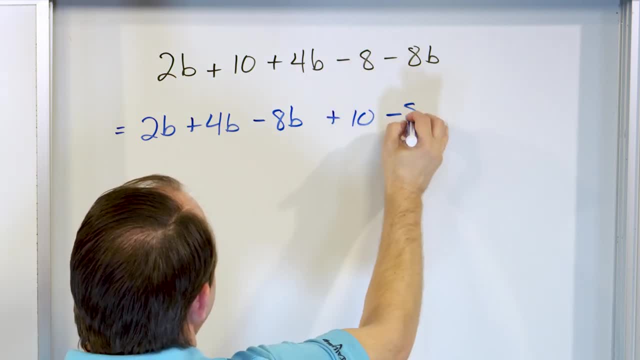 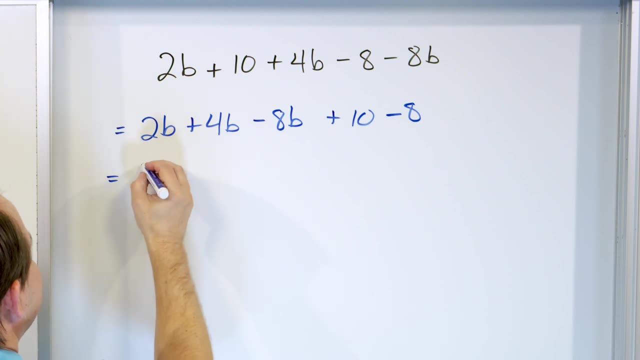 ten, And then we have the minus eight, And now we've grouped all our terms together that are the same, And all of these are the same, And so we just add the numbers together. What is two plus four, It's six. So we have six B. We still have to subtract eight here, And then we can add these. 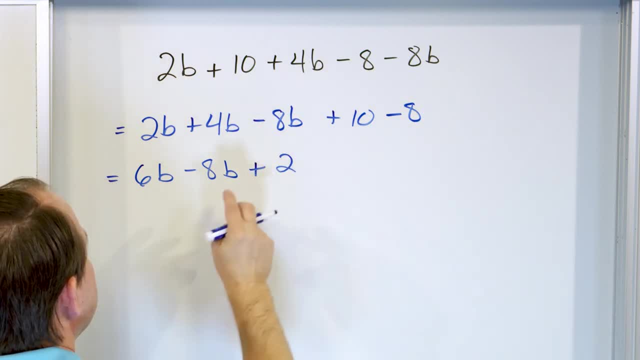 numbers anytime we want. Ten minus eight is going to be positive two. So we have six B minus eight, B plus two. Now these are of course like terms. You have six minus eight. What do you get? when you have six minus eight, You have negative two. Basically, you subtract and the sign goes with: 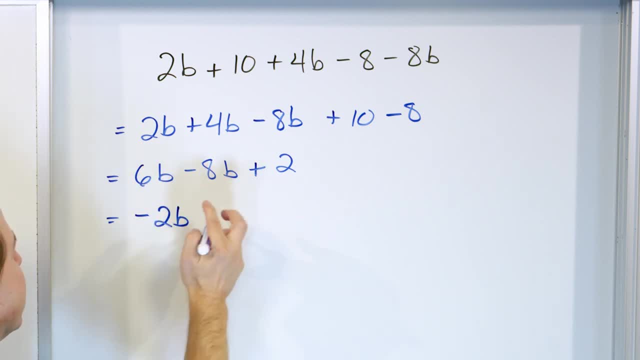 the larger absolute value. But there has to be a- B there, because these are like terms plus two, And you typically want to write the variable term first, which is exactly what we have: Negative two, B plus two, And that's the final answer. All right, Only I think two or three more. Let's take a look. 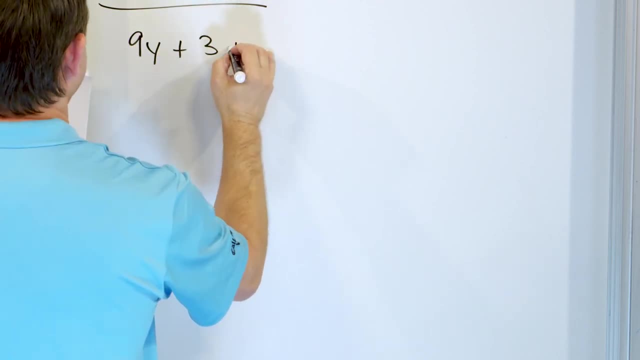 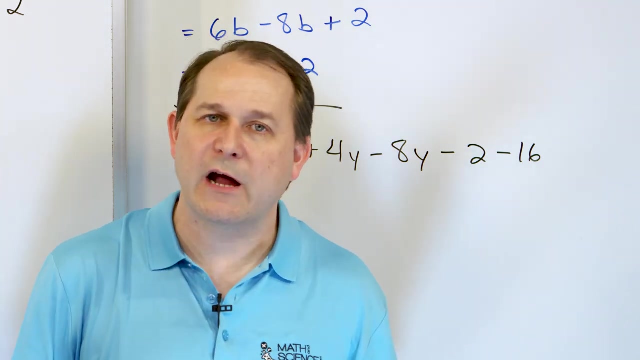 at nine times Y plus three plus four times Y minus eight times Y minus two minus sixteen. Now we can tackle problems. There are many ways to tackle problems. I could do this another way, but I want to take the opportunity to do it a slightly different way. 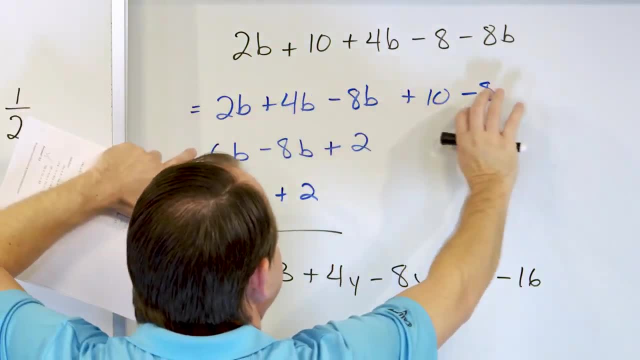 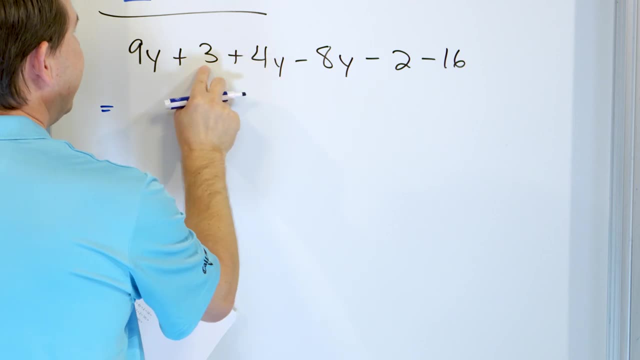 What we've usually been doing is rearranging everything so all the terms are together and then move along. But we don't have to do it that way. What you can do is recognize: OK, these are different, And of course these are different, But these here, they're already right. 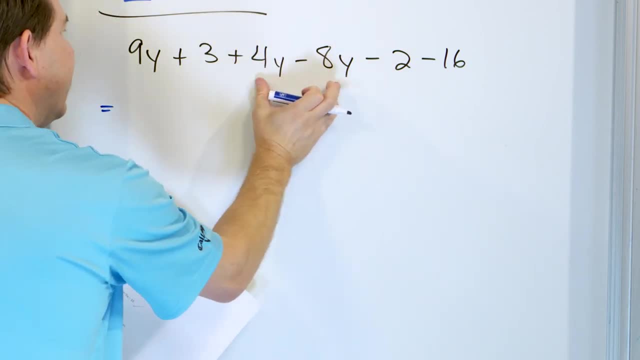 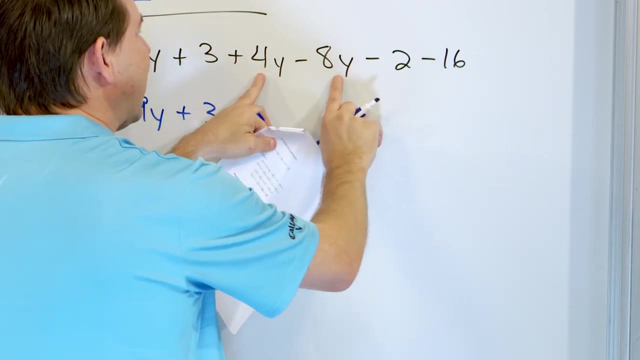 next to each other and they're already like terms, So we'll just do this first. Right, We have nine Y. We'll deal with that later. We have plus three. We'll deal with that later, But we can choose to subtract these first. What is four minus eight? Because the terms are the same. So we have: 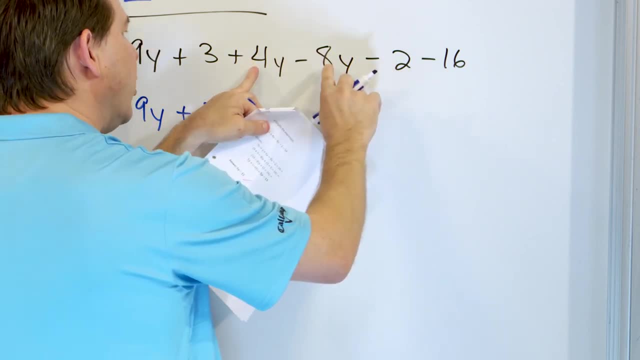 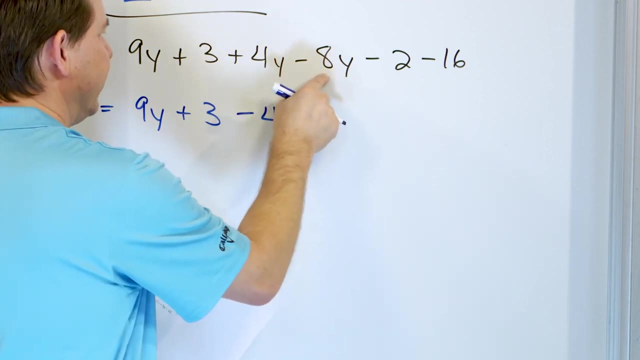 the terms are the same. We can just take four minus eight, And since it's a small number minus the big number, the answer will be four. But it really will be negative four, Four, negative four, Y, Four minus eight, or four plus a negative eight, if you want to think of it that way. Right, Because 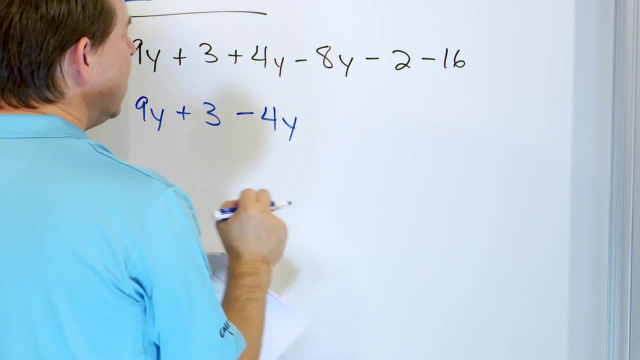 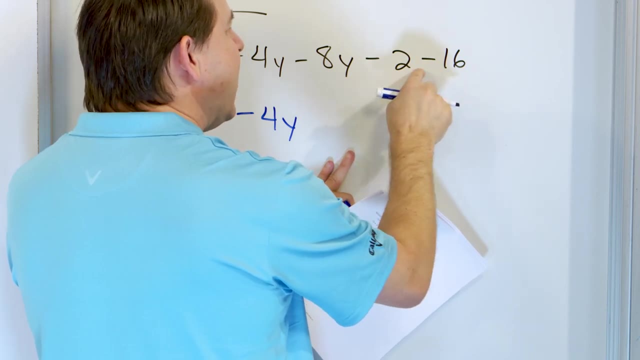 the sign goes with the larger absolute value of the eight there. And then what do we have here? We have two terms that are also alike. This is a negative two. You have to read this as negative two. And this is minus sixteen more. Remember you have a negative number subtracting more You have. 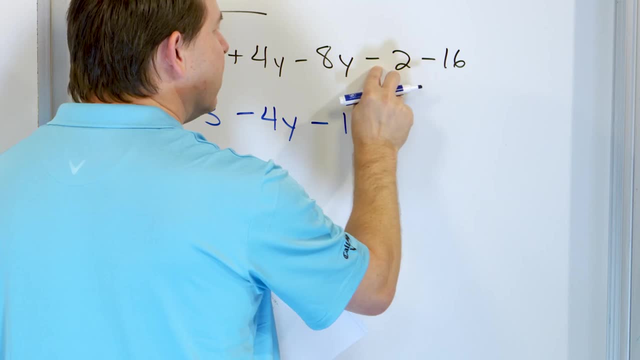 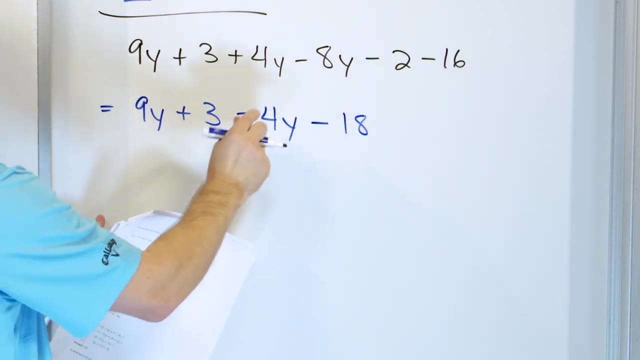 to add these, but it becomes a negative eighteen. If you have negative two dollars and I subtract sixteen more dollars, you are really in debt Eighteen dollars. So negative two minus sixteen. So what we did is because these were already next to each other. we would do that because these 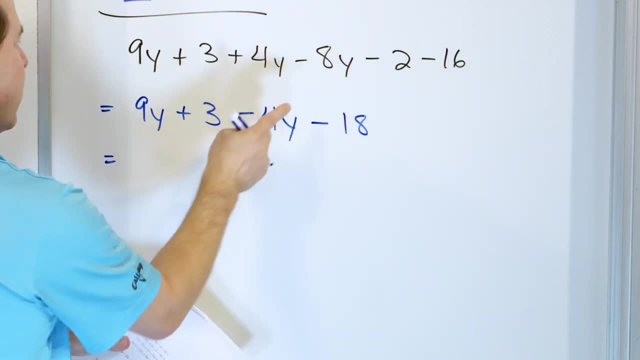 are already next to each other. We will do that, and then we can rearrange the smaller expression. We will have nine Y, This one goes right next next to negative. four Y, The negative sign comes with it. Plus three goes right here, and then minus eighteen goes right there. 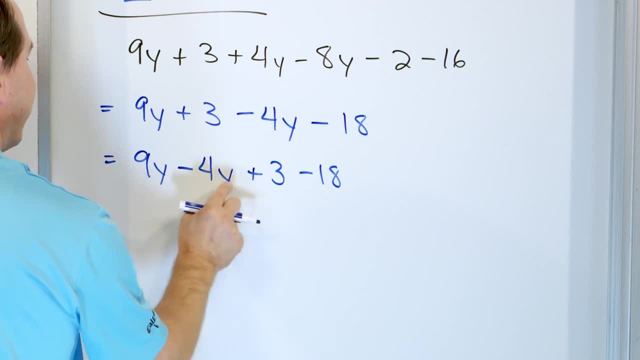 All right. So here we have like terms, We have Y terms. What is nine minus four? It is five, Five. what Five Y? It's nine hamburgers minus four hamburgers. I must have five hamburgers. And then, of course, 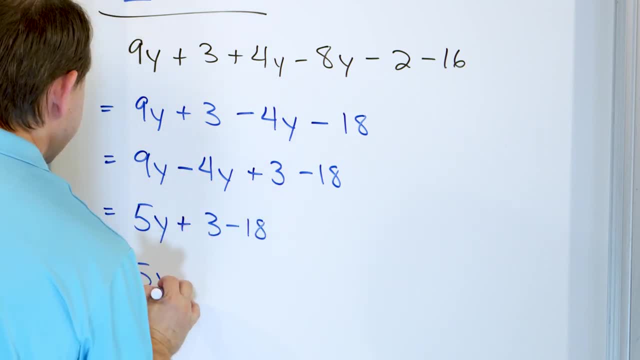 I have plus three minus eighteen And I have to deal with three minus eighteen. What do you do when you can't do the subtraction? You just subtract as usual. Eighteen minus three is fifteen, But then you make it negative because it's backwards Right, The sign goes with the larger. 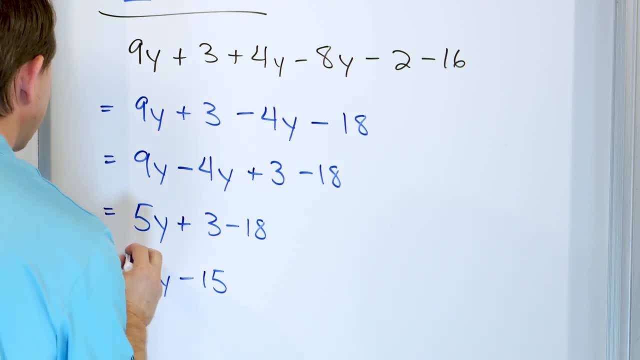 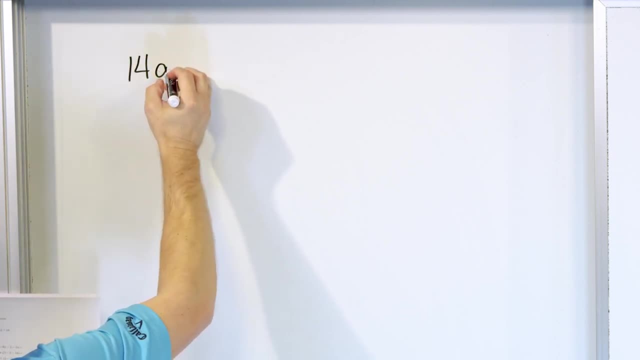 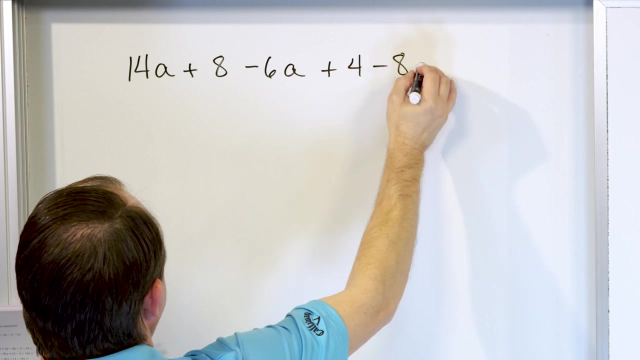 absolute value. So you have five Y minus fifteen. Five Y minus fifteen. That is the final answer. All right, Only two more problems. Let's take a look at fourteen A plus eight minus six A plus four minus eight A. All right, So I don't have any terms right next to each other that are like 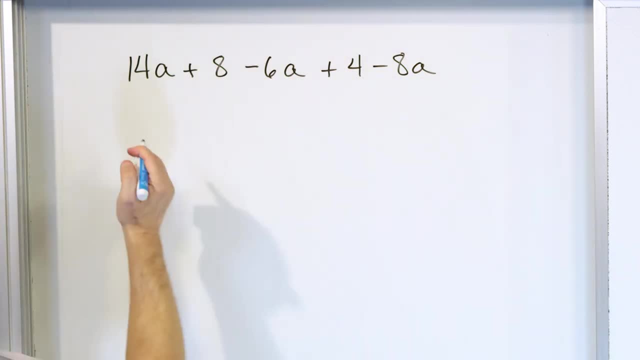 terms. So let's go ahead and just rearrange things as we've been doing. We start with 14 times A. Here is a like term. It has the same variable. The minus sign goes with it, So it's minus six A. 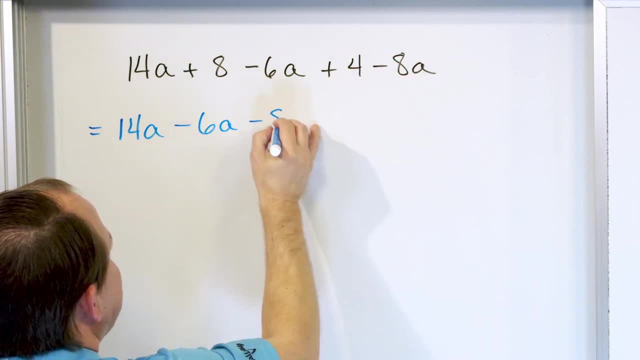 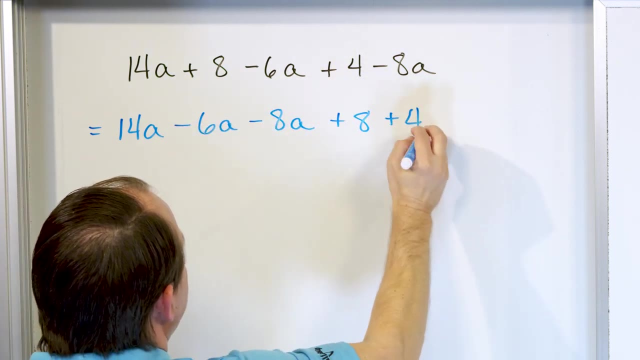 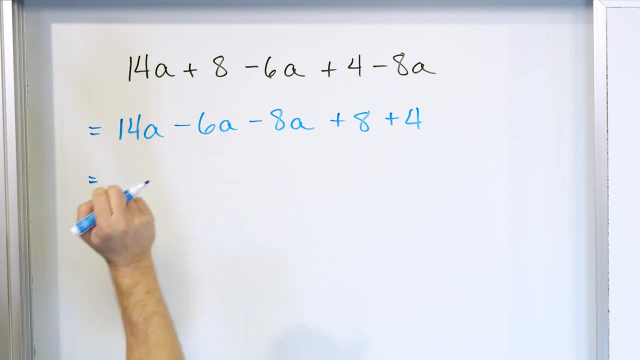 This is also a like term. The minus sign goes with it Minus eight A. And then we go back through and catch this term plus eight at the end, And this term the plus goes with it Plus four, And now all the terms are next to each other. And then we go left to right. What is 14 minus six? 14 minus? 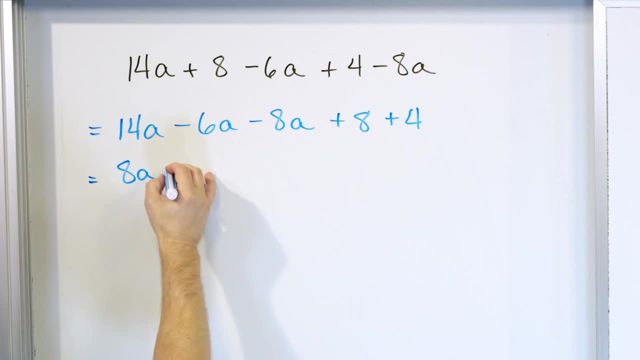 six is eight, So we write it as eight A. Rest of it, Let's just copy it for now: Minus eight A plus four. Next step: I have eight A minus eight A. What is what happens there? It's eight horses minus. 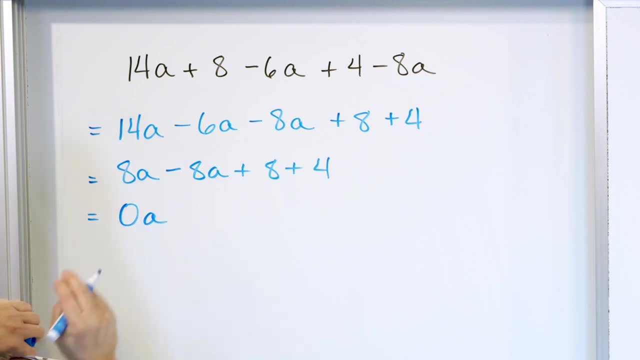 eight horses. Well, you don't have anything left. You have zero horses, Zero A Right. And let's go ahead and add these. Eight plus four is 12.. So, plus 12, because it's positive. eight plus four more is positive 12.. Now, what is zero times A? Remember, A can be a number, but zero times. 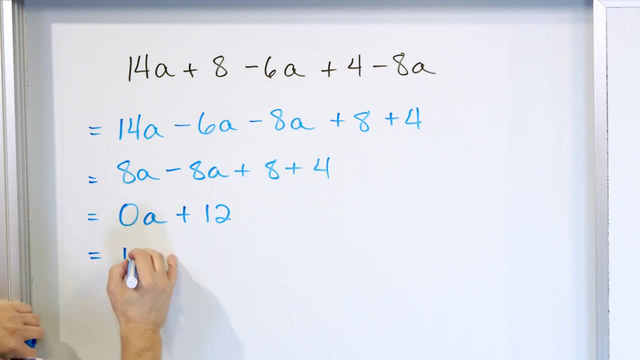 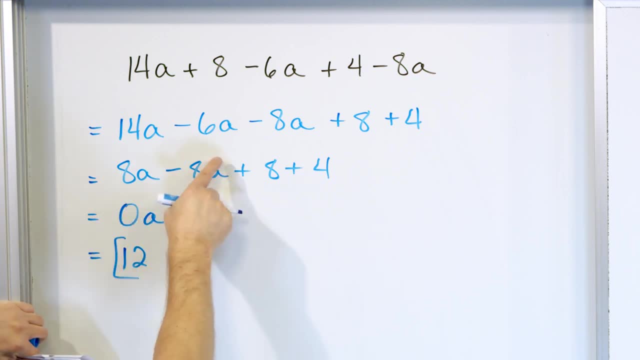 really the final answer, because this term eight A minus eight A, it just gives you zero. And then the answer you have, 12- has no variable at all. And the reason is because if you take 14 minus six minus eight, it turns out that there's no horses left, for lack of a better word: The variable term. 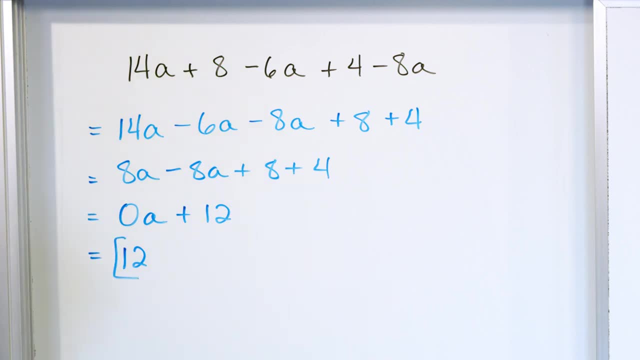 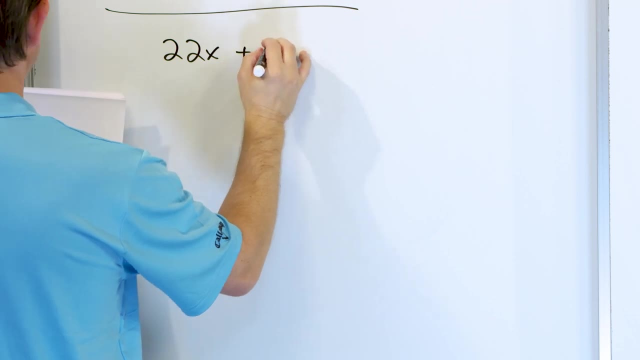 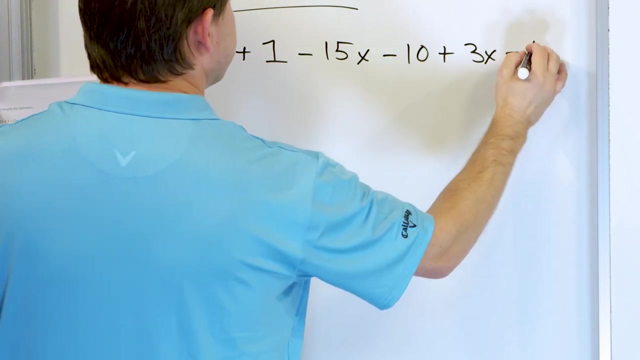 drops away. All right, Last problem. Last problem, Let's take a look at 22 times X plus one minus 15 minus 10 plus three times X minus four, Just like this. Now, again, I don't see any pairs of terms. 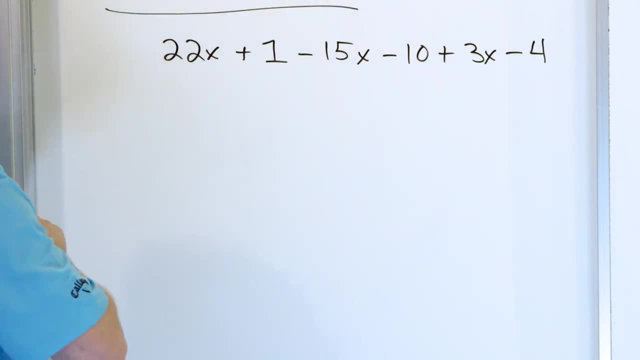 that are like terms sitting right next to each other. So let's go ahead and just rearrange everything And we have 22 X right here. This is a like term because it has an X to the first power. Same as this. The minus sign comes with it: Minus 15 X. This is a like term, plus three X. 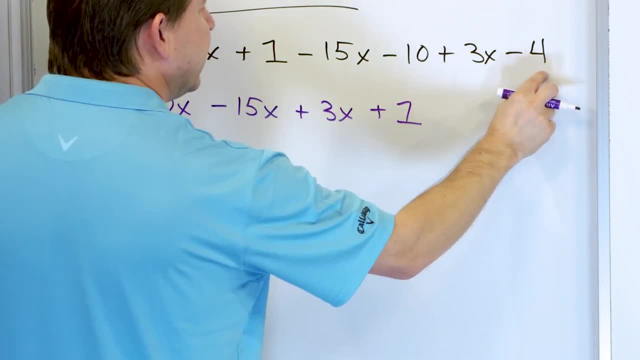 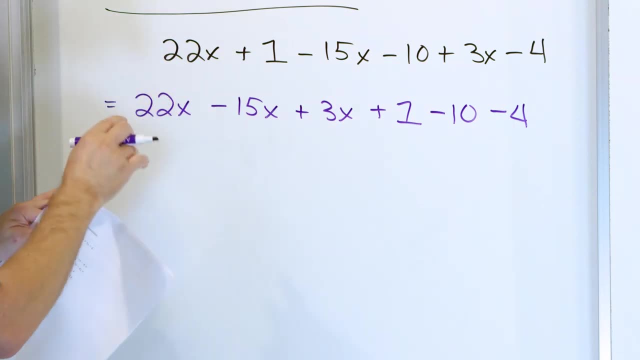 The plus one is a different term, but I'll group it with the minus four, right? Or actually there's a minus 10 that comes down here and then a minus four. So really all I did was write the same terms down in a different order, where the variables are all. 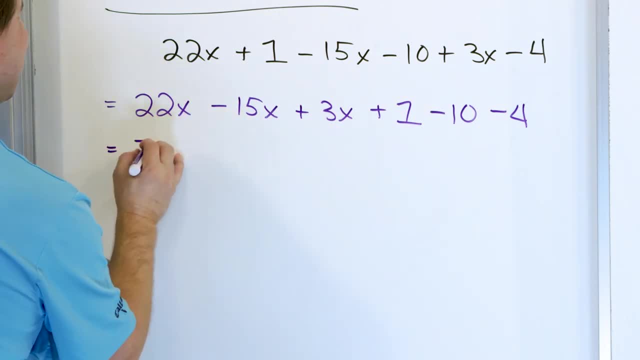 the same here: 22 minus 15 is seven. but it's not just seven, It's X's minus X's, So seven X's here. We'll add the three X later, And then we'll deal with the numbers later too. Let's just deal with. 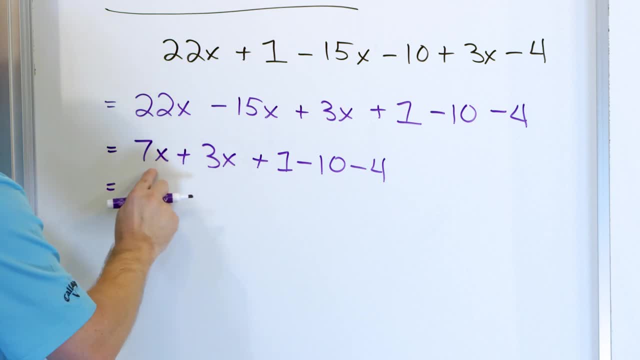 all that later Here, seven X plus three X. These are like terms. They make 10 X. So it's like seven rabbits plus three more rabbits. Yeah, 10 rabbits. Right now let's start dealing with the numbers. What is one minus 10?? You can't really. 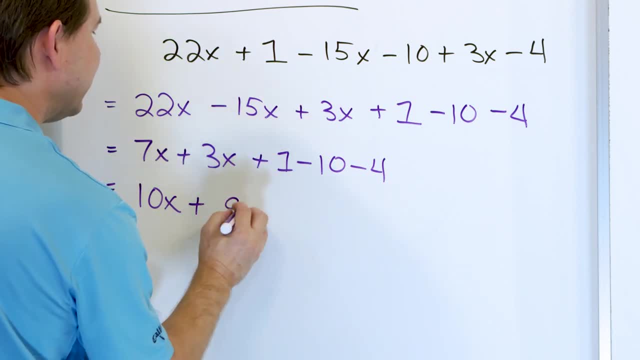 do that subtraction right. So just subtract as normal: 10 minus one is nine. but the sign goes with the larger absolute value, the negative here. So really it becomes minus nine. So we'll just erase that plus sign. The answer to this is negative nine. We still have to subtract that. 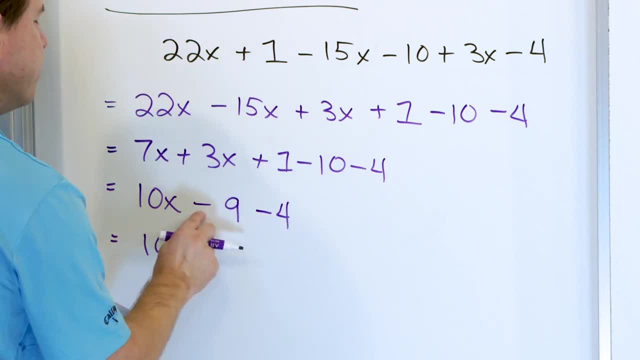 four. So we have 10 times X. What is negative? nine minus four. We go deeper, negative and you get to negative 13. So you, essentially, we add these and make it negative, So you get 10 X minus 13. And now you can see why it was so. 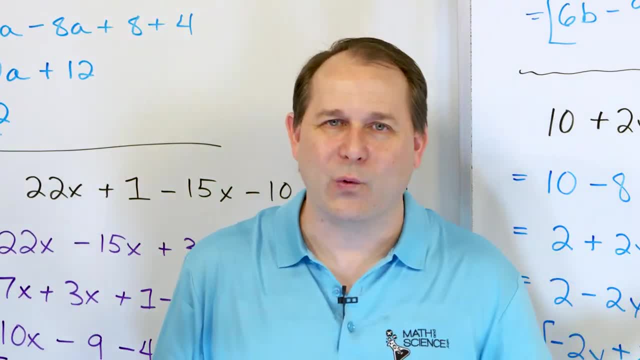 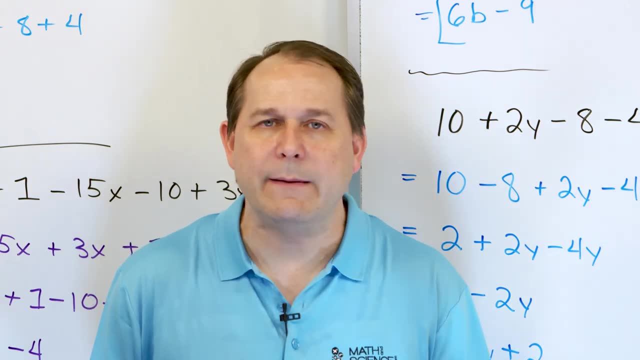 critical that we master the idea of adding and subtracting integers from before. We did a whole entire lessons. We just learned how to add and subtract negative and positive numbers and it gets kind of boring to do it. But now you see why: because we're combining that with the idea of